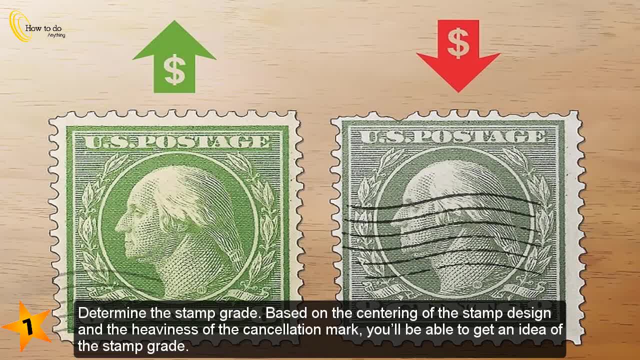 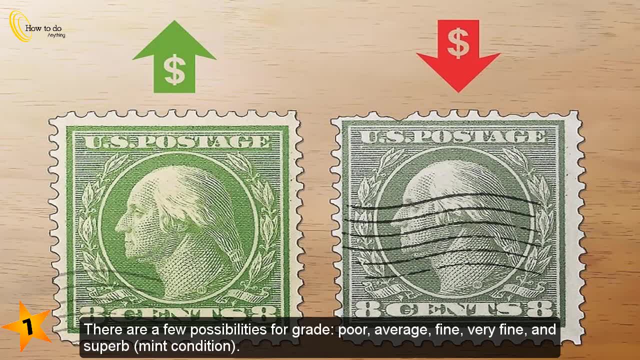 Based on the centering of the stamp design and the heaviness of the cancellation mark, you'll be able to get an idea of the stamp grade. There are a few possibilities for grade: Poor, average, fine, very fine and superb mint condition. 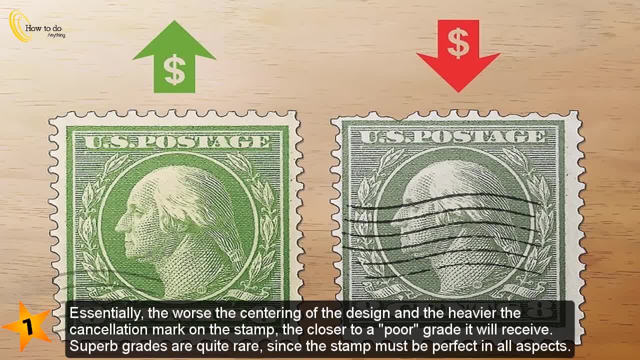 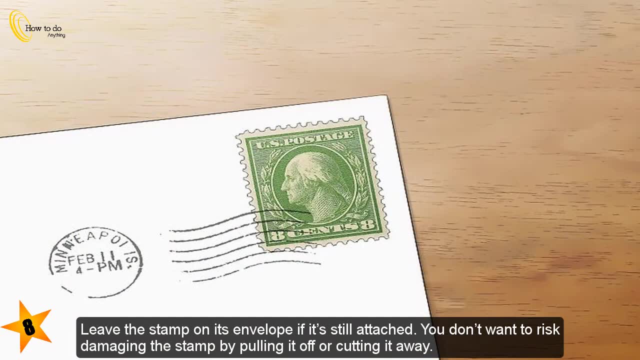 Essentially, the worse the centering of the design and the heavier the cancellation mark on the stamp, the closer to a poor 8.. Leave the stamp on its envelope if it's still attached. You don't want to risk damaging the stamp by pulling it off or cutting it away. 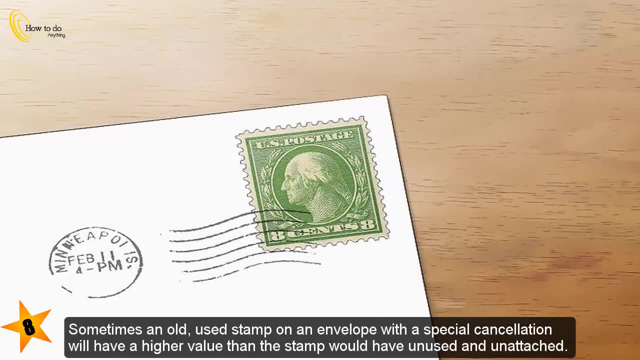 Sometimes an old, used stamp on an envelope with a special cancellation will have a higher value than the stamp would have unused and unattached. Ask an expert at a stamp show or get a professional appraisal to see if the stamp should be removed. Part 2. Determining History and Rarity. 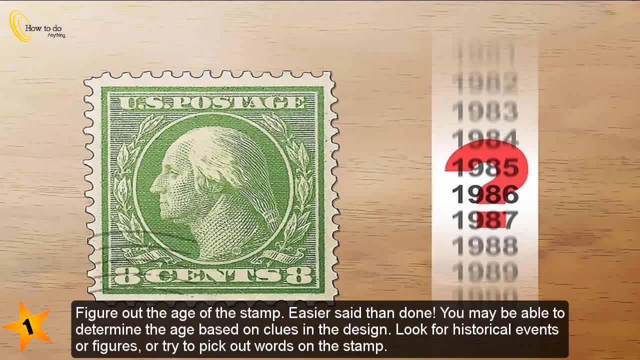 1. Determine the stamp's history and rarity. 2. Determine the stamp's history and rarity. Figure out the age of the stamp. Easier said than done, you may be able to determine the age based on clues in the design. Look for historical events or figures, or try to pick out words on the stamp. 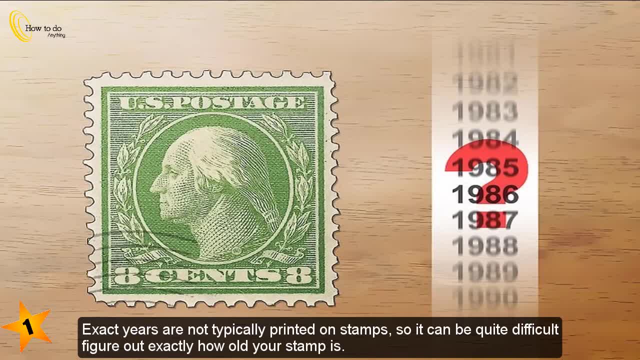 Exact years are not typically printed on stamps, so it can be quite difficult figure out exactly how old your stamp is. Head to an expert stamp dealer if you need extra help. The older the stamp is, the more valuable it will be, so it's worth the extra effort. Stamps printed within the last. 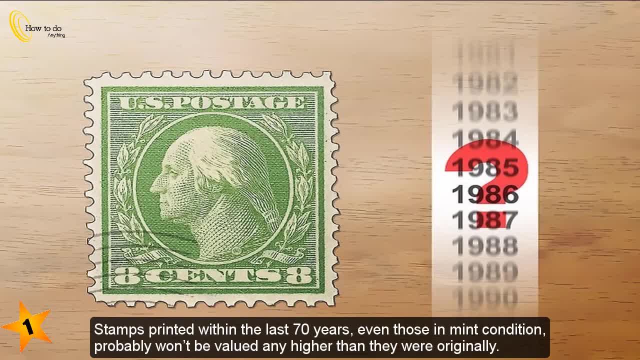 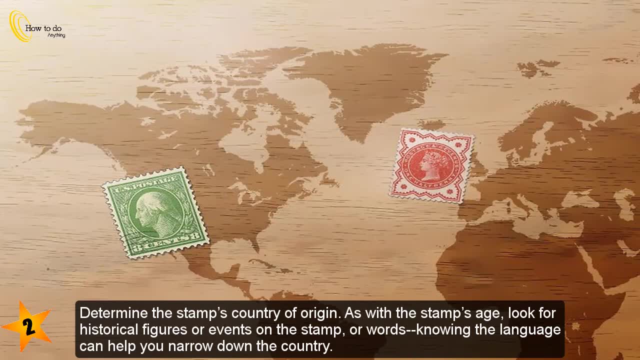 70 years, even those in mint condition. 2. Determine the stamp's country of origin. As with the stamp's age, look for historical figures or events on the stamp or words. knowing the language can help you narrow down the country. A picture of Queen Victoria, for example, is probably from 19th-early-20th-century. 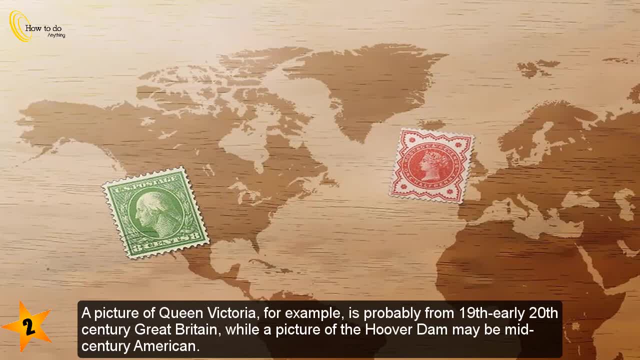 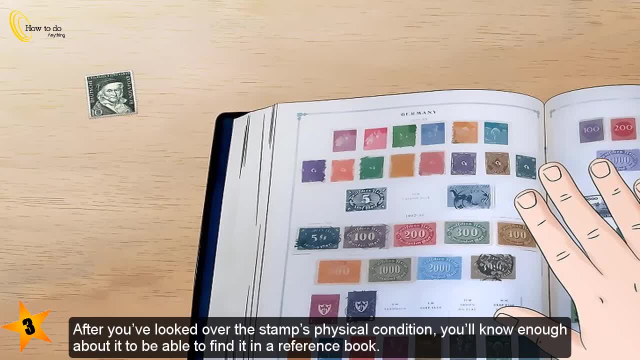 you may want to start with a reference book. You may want to start with a reference book to determine the age and country of origin. After you've looked over the stamp's physical condition, you'll know enough about it to be able to find it in a reference book.